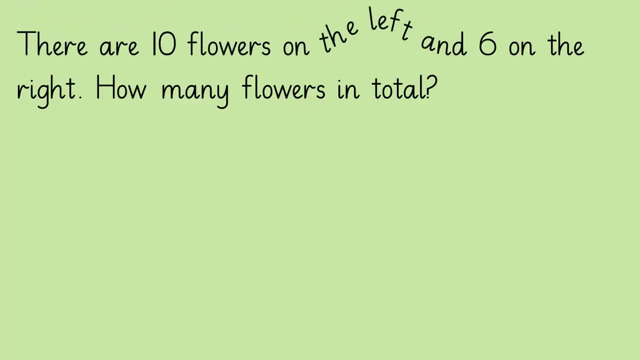 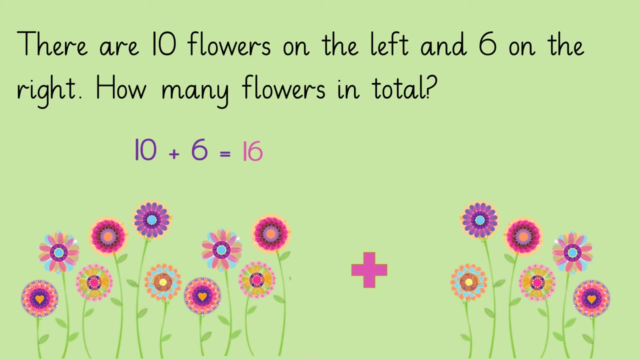 Children. let's learn about word problems with the help of few examples. There are ten flowers on the left and six on the right. How many flowers in total? Ten plus six? Keep ten in your mind and count six more Correct students, It makes sixteen. Let's check our answer with the help of the pictures. 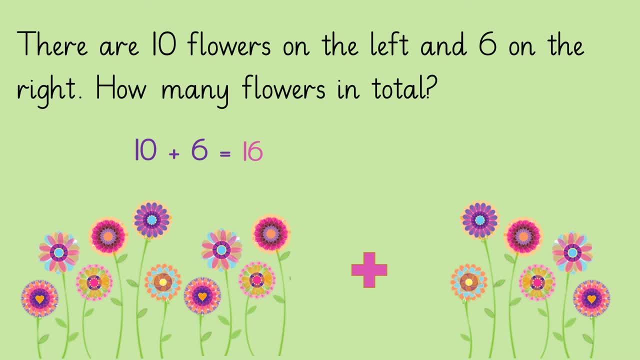 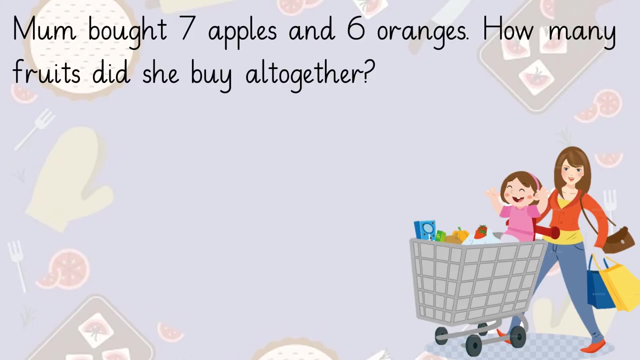 You can see ten flowers on the right left-hand side and six on the right. yes, there are 16 flowers in total. hmm, yummy, who likes fruits? mum bought seven apples and six oranges. how many fruits did she buy all together? so, students, seven plus six means keep seven in your mind, and 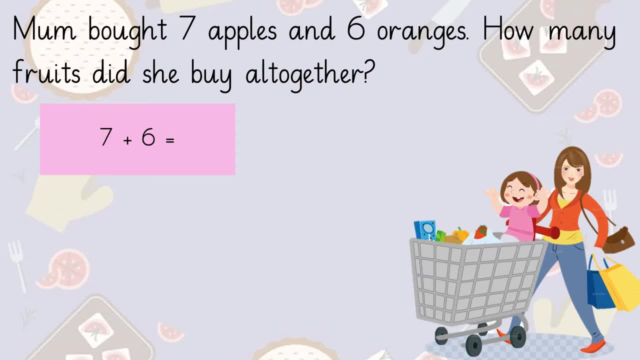 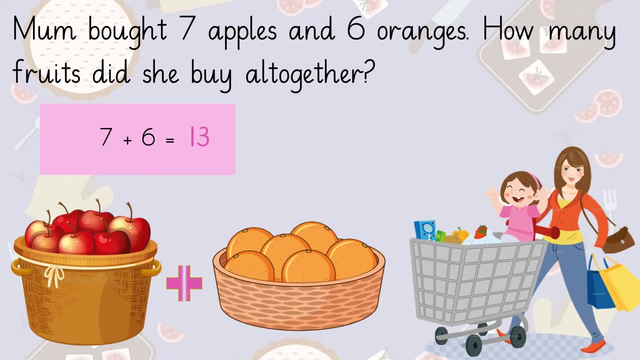 count on six well done students, it makes 13. let's confirm it with the help of the pictures. you can see seven apples and six oranges in the baskets. so mum bought seven apples and six oranges in the baskets. so mum bought seven apples and six oranges in the baskets. so mum bought. 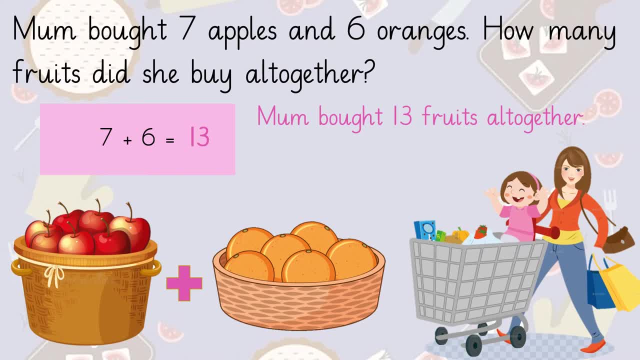 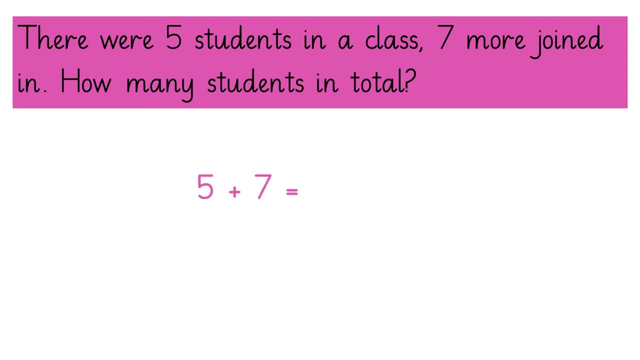 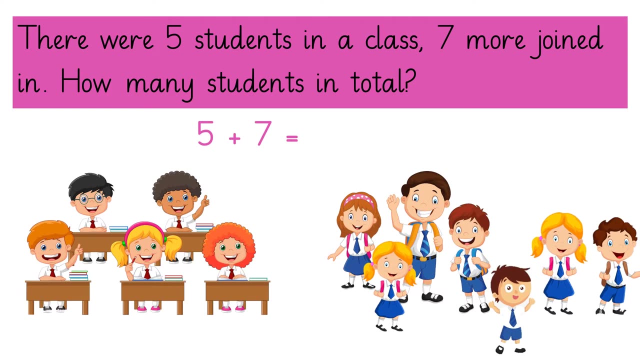 thirteen fruits. all together, there were five students in our class. seven more joined in. how many students in total? children? let's count with the help of the picture: 5 plus 7, it makes 12. there are 12 students all together. students: let's count with the help of the picture: 5 plus 7, it makes 12. there are 12 students. 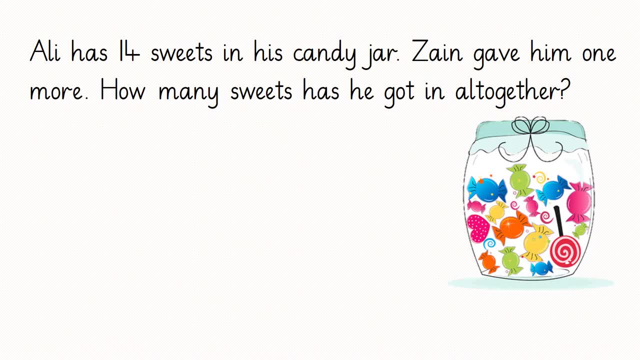 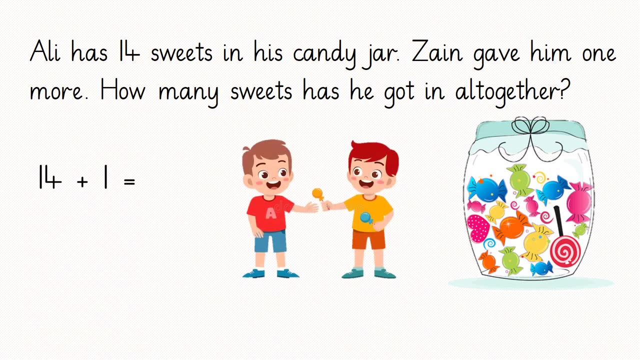 let's practice. the last example: Ali has 14 sweets in his candy jar. Zan gave him one more. how many sweets has he got in all together? children, you can see 14 sweets in the jar. hmm, that's so simple. just add 1 into 14, so you will. 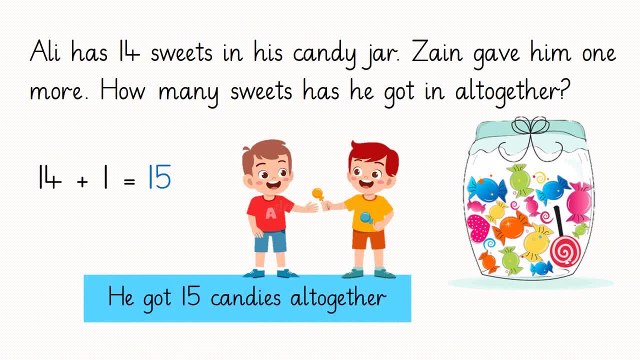 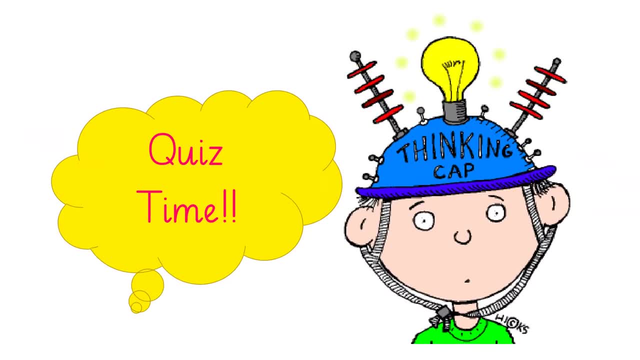 get 15. yes, Ali has 15 sweets in his candy jar. Zan gave him one more. how many sweets has he got in all together? children, you can see 14 sweets in the jar. keep your thinking caps on and remember. you can pause the video to answer.